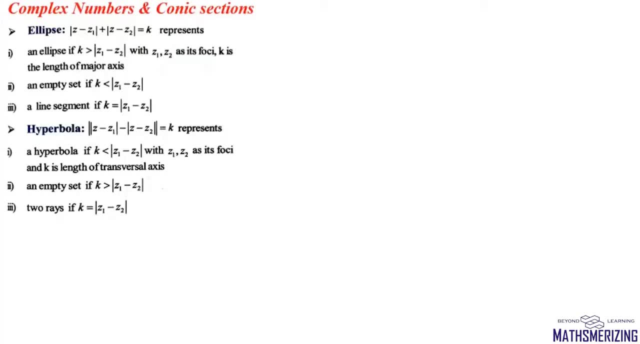 In this video we will be discussing how to represent equation of conic sections in complex numbers. Now, in complex numbers, what we know is: any modulus is nothing but distance between two points. Say, if we have two points, z1 and z2, and there are points a and b, then this distance 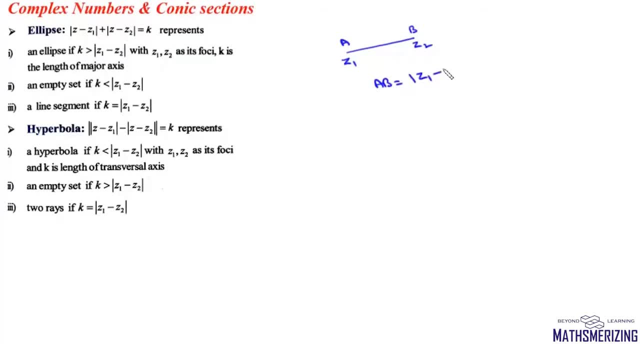 it is represented by mod of z1 minus z2. So in complex numbers, any modulus, it represents distance between two points. Now we can write equation of an ellipse using focal property of ellipse. So if we have any ellipse whose focus is at say, z1 and z2, then we know that. 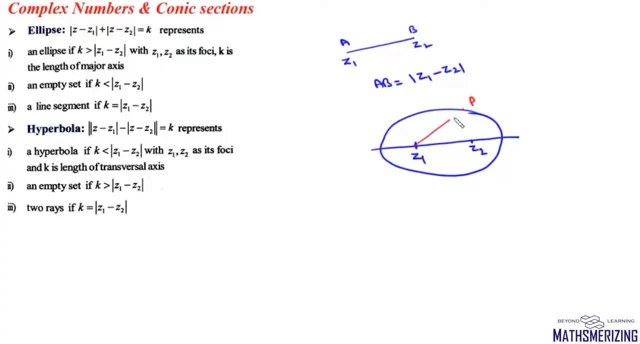 sum of distances of any point on ellipse from the two focus is equal to its length of major axis. So suppose this is s1 and this is s2, then we can write ps1 plus ps2 and it is equal to 2a, which is length of major axis. Now suppose this point p is z. now we can write this distance ps1. 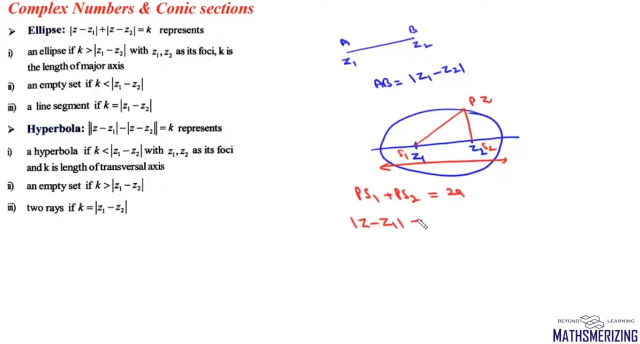 as mod of z minus z1.. In the same way, we can write ps2 as mod of z minus z2 and it is equal to 2a. So this is how we can represent equation of an ellipse in complex numbers, where distance between z1 and z2, it is distance between two focus and it will be 2ae. 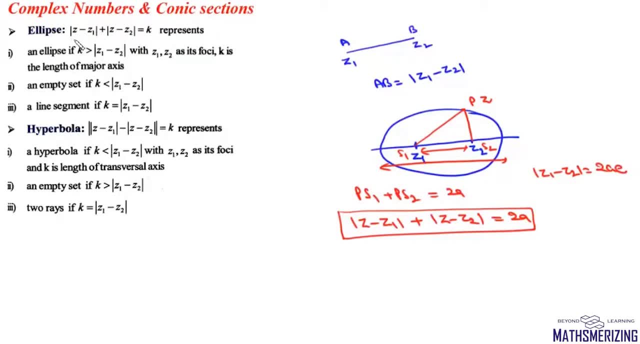 Any equation which is of the form mod of z minus z1 plus mod of z minus z2 equals to k. it will represent an ellipse if k is greater than mod of z1 minus z2.. Now, in this case, k is 2a and. 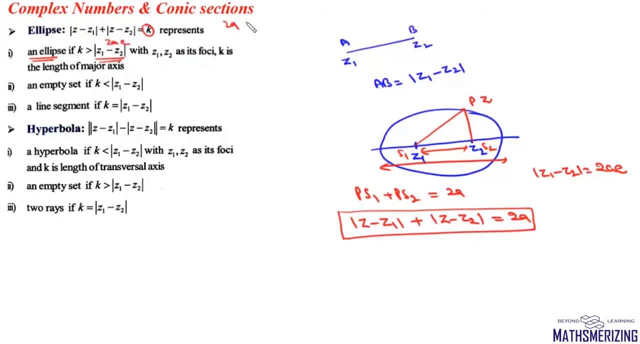 z1 minus z2 is 2ae, So 2a should be greater than 2ae, so that e should be less than 1.. If k is less than 1, then we can represent any locus. Now, what if k is equal to z1 minus z2.. So if we have this, 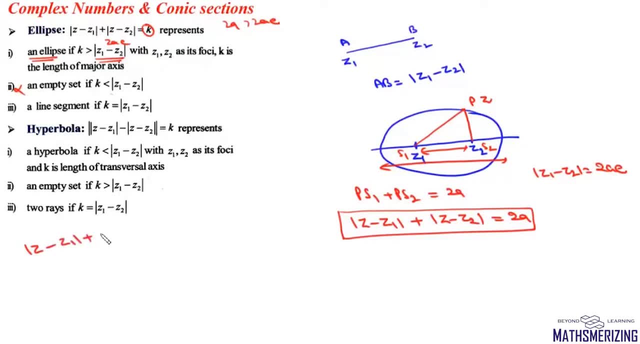 condition: when we have mod of z minus z1 plus mod of z minus z2 and it is equal to mod of z1 minus z2, then if z is p, z1 is a and z2 is b, then we can write pa plus pb. it is equal to ab, which is: 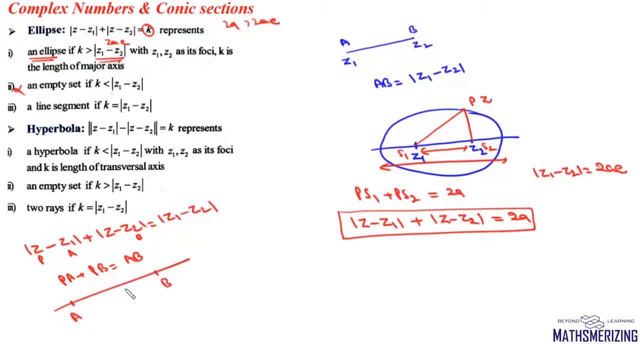 nothing but condition of collinearity. So in this case pa plus pb can only be equal to ab if p lies between a and b. So in that case it will represent this line, segment ab. In the same way we can use focal property of hyperbola to represent its equation in complex numbers. So suppose now we have any. 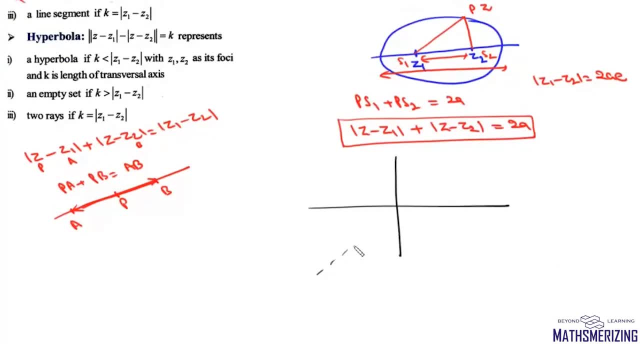 hyperbola whose focus is at z1 and z2, and then we have a point p on this hyperbola. then focal property of hyperbola says difference of distance from the two focus of any point on hyperbola must be equal to 2a. So from here we will get this condition that ps1 minus ps2 and its modulus it. 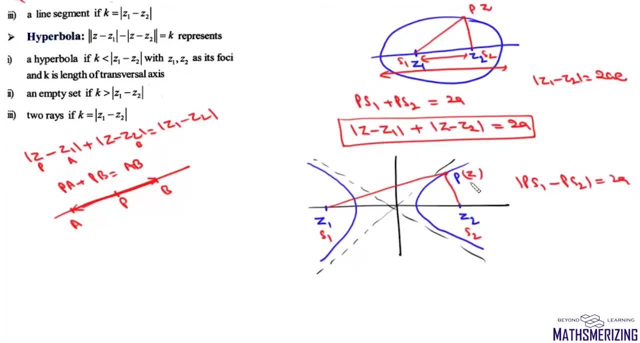 must be equal to 2a. Now, ps1 is nothing but distance of p from s1. So it will be mod of z minus z1 minus ps2 is mod of z minus z2 and it must be equal to 2a. 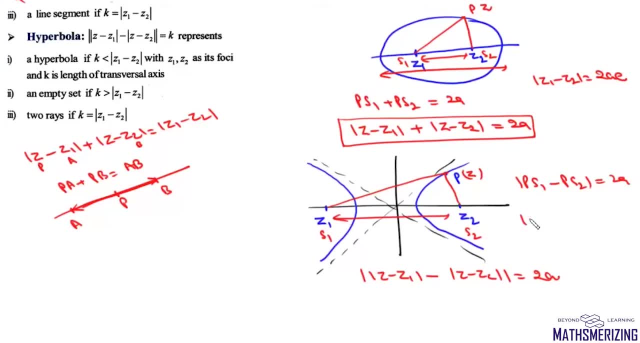 Now again for hyperbola. also, distance between focus, that is, mod of z1 minus z2, is 2ae. So we get this condition that if mod of z minus z1 minus mod of z minus z2 is equal k, it will represent a hyperbola if k is less than mod of z1 minus z2.. Now in this case, 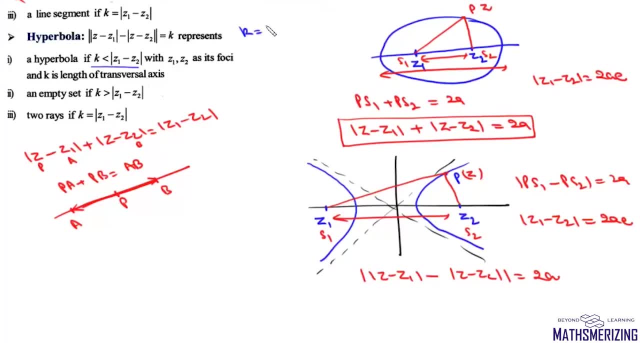 k is again 2a and it will be less than 2ae, since for hyperbola, e is greater than 1.. So this k, it should be less than mod of z1 minus z2.. If k is greater than mod of z1 minus z2, 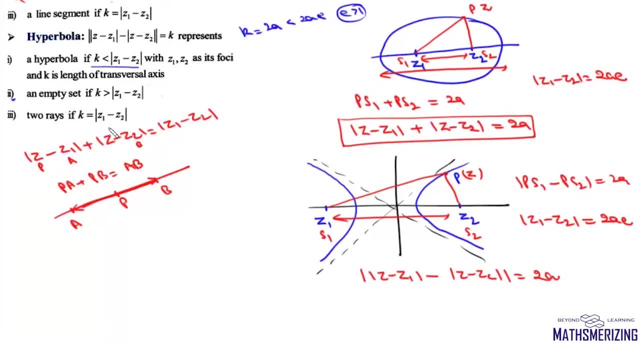 it represents an empty set. and if k equals z1 minus z2, then we will have this condition, that mod of z1 minus mod of z2 whole mod, and it is equal to mod of z1 minus z2, which is p-p, which again will be a condition of collinearity. 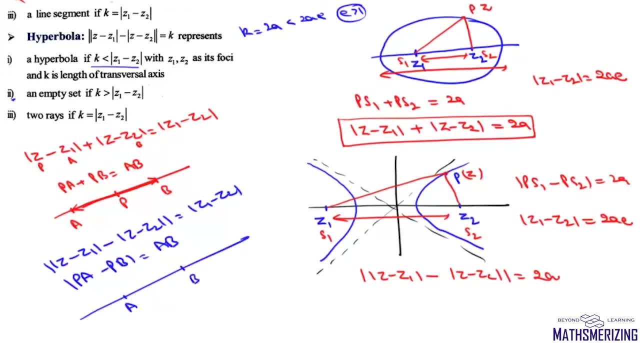 So we have two points, a and b, The this point p. It must lie around on this line there joining AB, except for the points on this line, segment AB. So this is how we represent equation of ellipse and hyperbola in case of complex numbers. 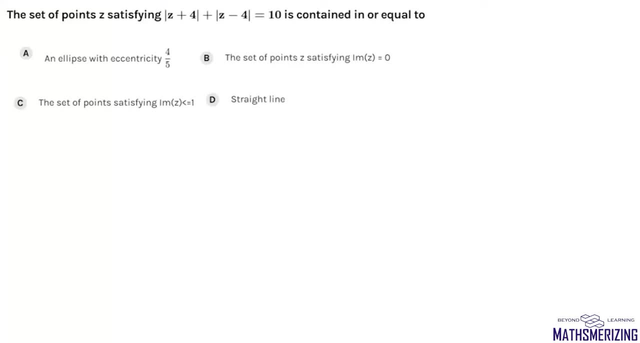 Now let us take a problem. it says the set of points z satisfying mod of z plus 4 plus mod of z minus 4 equals 10 will represent which of the following locus? Now, if we look at this equation, this is mod of z minus z1 plus mod of z minus z2, and it: 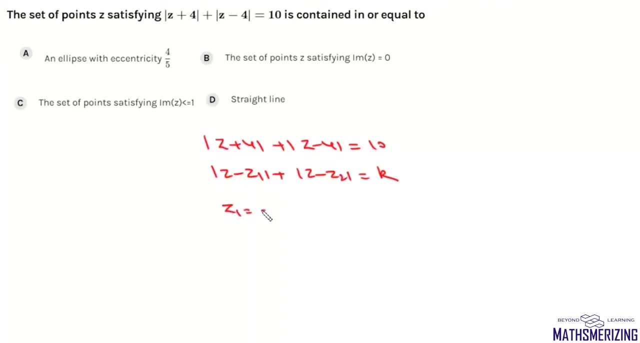 is equal to k. Now, in this case, z1 is minus 4, z2 is 4 and this is 2a and 2a is 10.. Now we will find mod of z1 minus z2,. mod of z1 minus z2 is 8.. 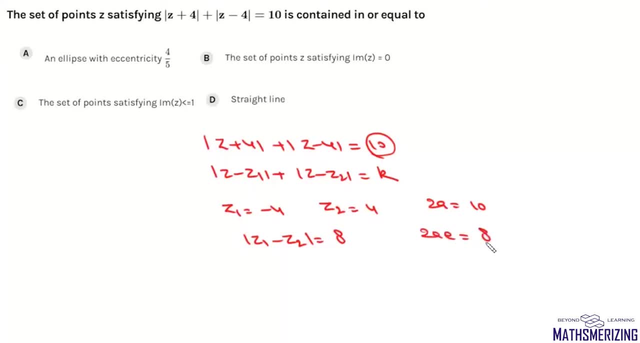 So 2aE, it is 8, which is less than k, which in this case is 10.. So if we will divide these two equations, we will get E as 8 by 10 or 4 by 5.. So this locus, it represents an ellipse whose eccentricity is 4 by 5, and that is your option. 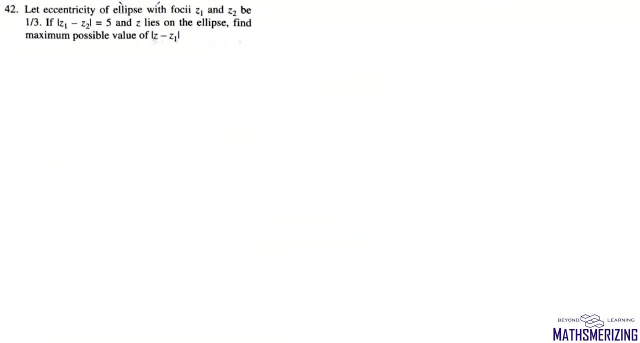 A. Now the next question is: let eccentricity of ellipse with foci z1 and z2 be 1 by 3.. So we have an ellipse whose eccentricity is 1 by 3.. If mod of z1 minus z2 is 5, that means distance between focus is 5..